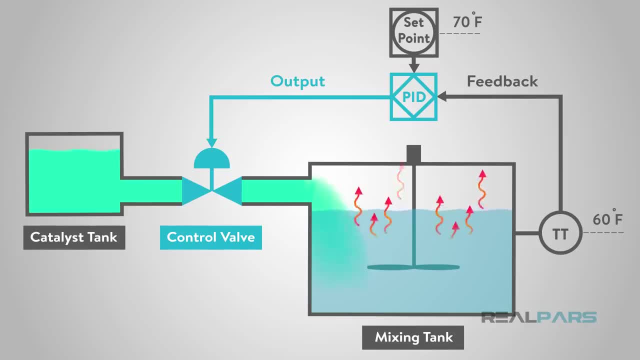 to be applied to a process so as to drive a measurable process variable towards the desired setpoint value. The controller uses an actuator to affect the process and a sensor to measure the results. Often, automation technicians and programmers are required to become familiar with configuring and tuning a PID loop control instruction. 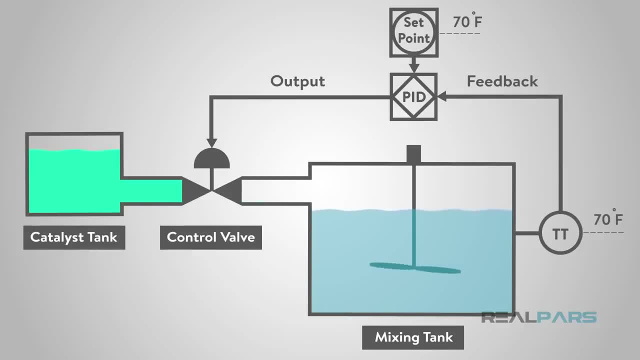 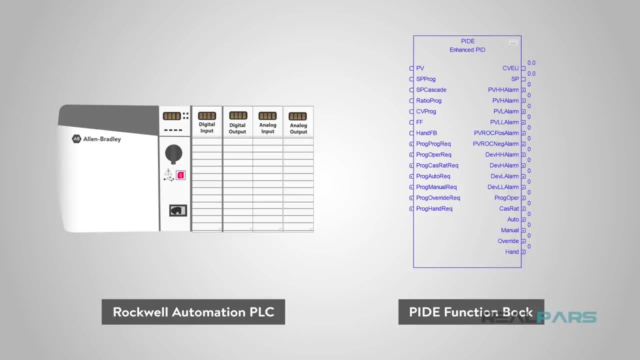 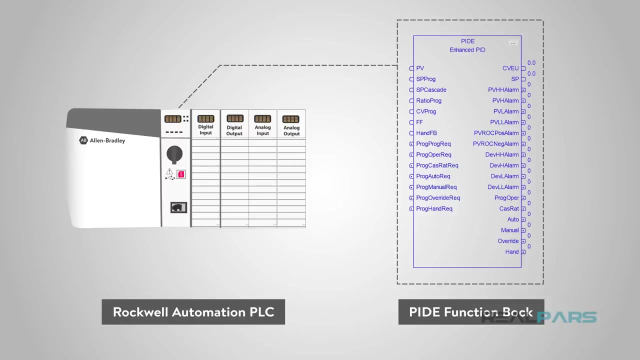 and it can be one of the most overwhelming when it comes to PLC programming topics. In this lesson we will discuss how a Rockwell Automation Control Logix 5000 PLC using the Enhanced PID Controller Function Block instruction PIDE. The PIDE is an Allen-Bradley Logix 5000 Process Automation Controller. 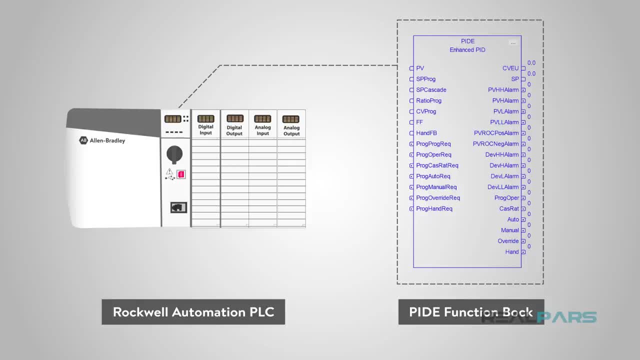 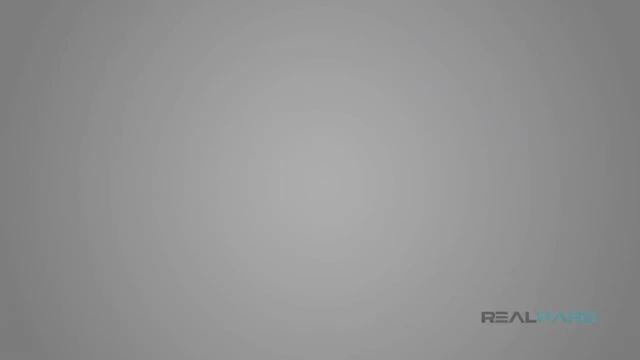 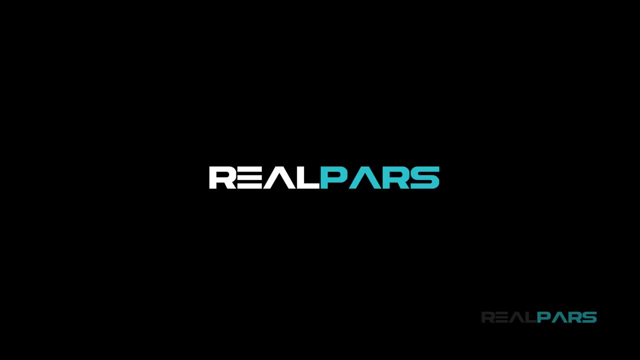 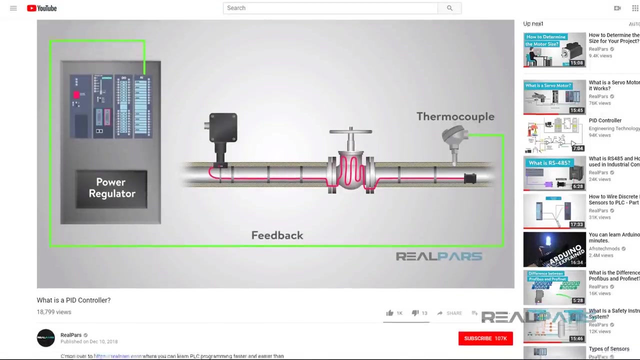 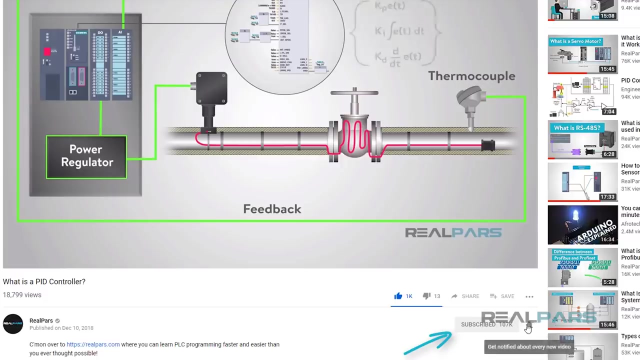 or PAC, family Control Logix and Compact Logix function block that improves on the standard PID found in all their controllers. Before we get started on today's video, if you love our videos, be sure to click the like button below. Then make sure to click subscribe and the little bell to receive notifications of new RealPars videos. 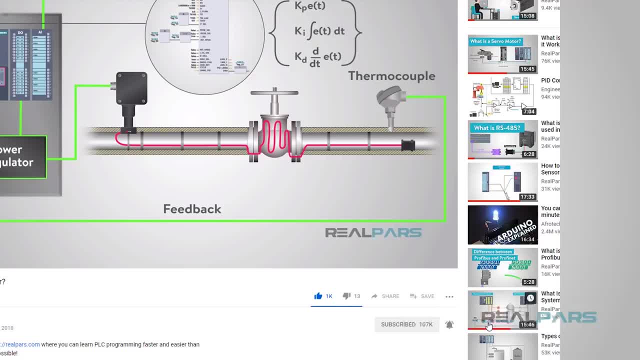 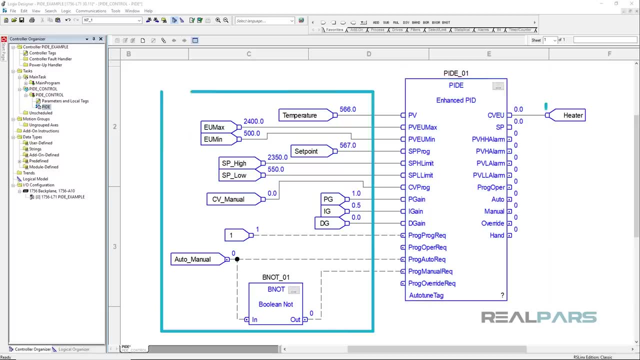 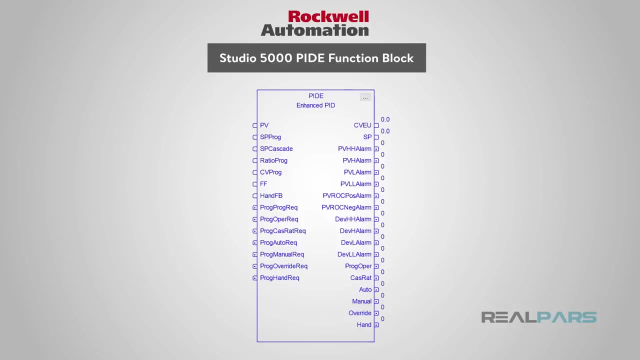 This way, you never miss another one. Function block programming uses diagrams with symbols to represent function and input and output connections between functions. While at first this function block can be quite intimidating, It shares similarities of the standard PID instruction and you'll only need to turn on parameters required by your control program. 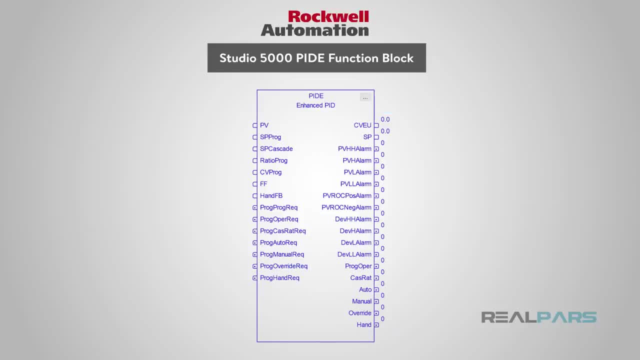 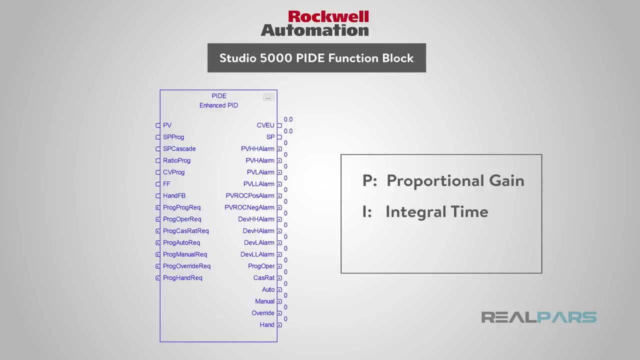 In this example, we will basically get you off the ground using the PIDE instruction and the program options essential to get it working. In case you may have forgotten what PID stands for: the P stands for Proportional Gain, I for Integral Time and D for Derivative Gain. 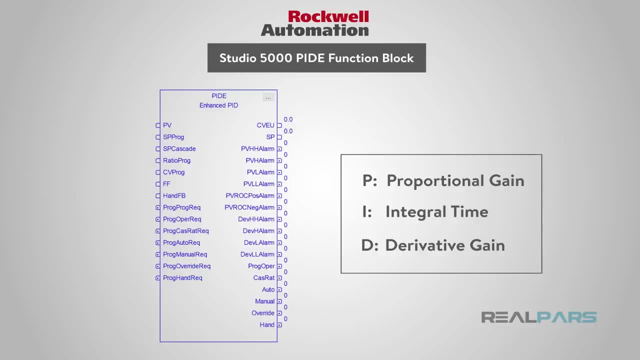 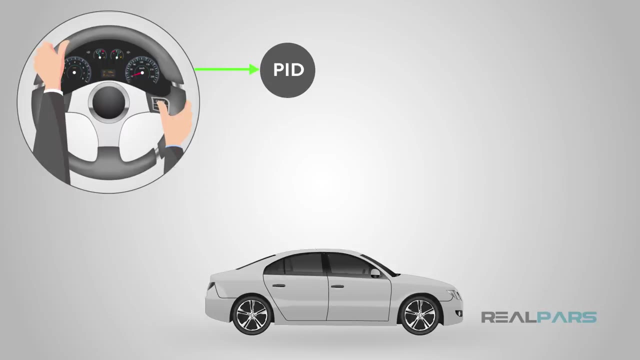 PID and PIDE are used for process control, which includes the automatic control of systems such as temperature, flow rate, pressure and speed. The cruise control on a car is a good example of this type of control. Basically, you tell the car to turn on the control. 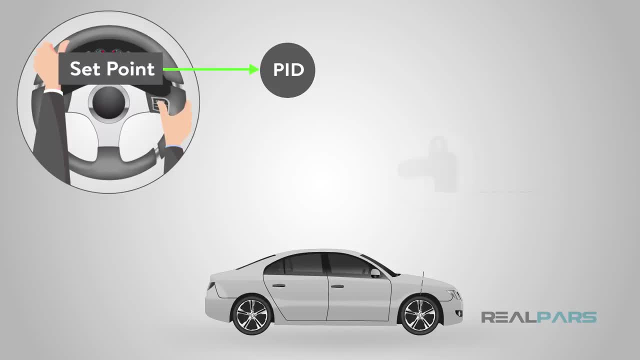 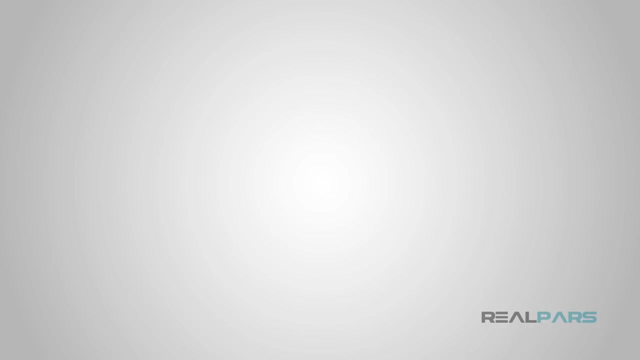 and you tell the controller how fast you want to go, The setpoint, and the controller samples the actual speed, the process variable, and then the controller calculates an output value, the control variable, and sends that signal to the gas pedal And, just as a PID, functional refresher. 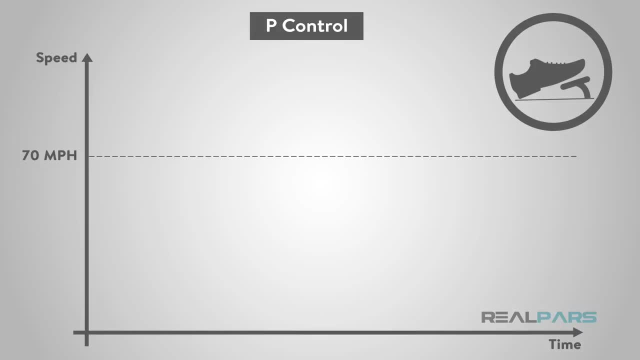 and using the car cruise control as an example. the P, or proportional, is described as in the farther you are from the desired speed, the more you press the gas pedal and, on the other hand, the closer you are, the less you press on it. 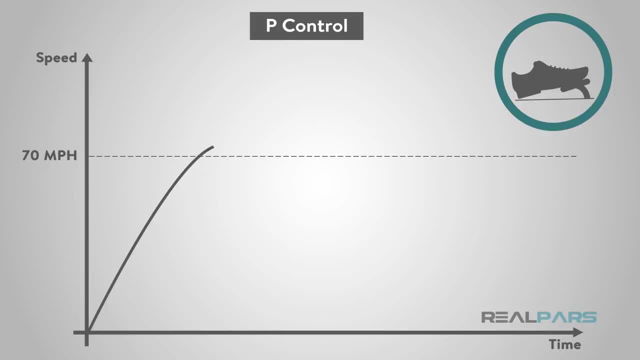 This works well, but when you get at the desired speed based on this rule, you would let off the gas completely And the end result is your car slows down and stays a little below the desired speed. Proportional control is the main ingredient of any control. 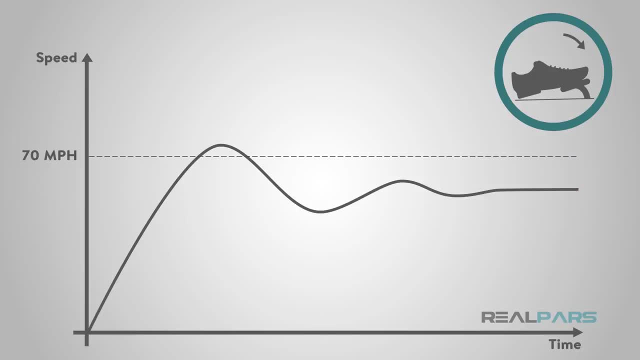 but may be a little inaccurate- For I or Integral. you wait for a little, and if there's no improvement you push a little more on the pedal. If you are stuck below the desired speed for a long time without progress, you push the gas pedal a little further. 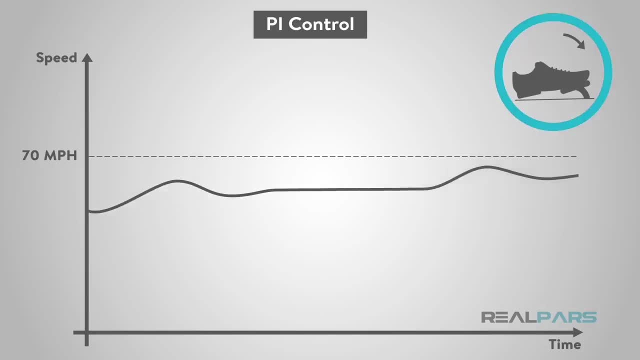 If you still do not make it to the desired speed for some time, you again push the pedal a little further down. Once you get to the desired speed, you leave the pedal where it is. Integral control gives you accuracy, but you have to wait. 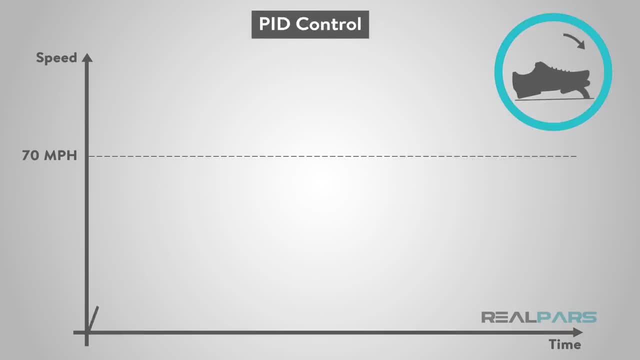 And for D or Derivative, you react to sudden changes. Let's say, a strong wind gust pushes your car Suddenly your speed surges fast upward toward the desired speed. You become startled so you release the gas pedal As the speed surge ends and the speed stabilizes. 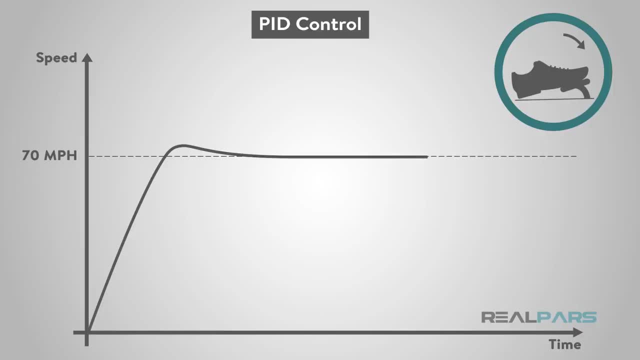 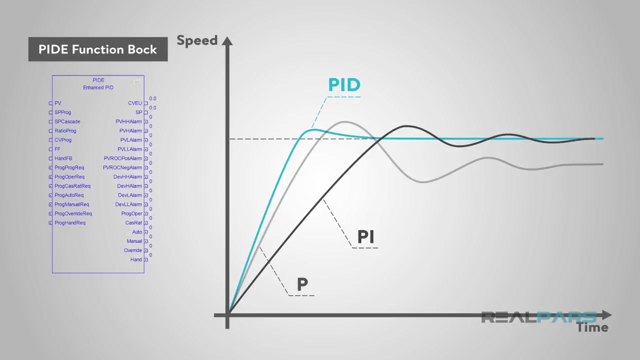 you will then return the pedal to where it was. Derivative control manages sudden surges and may provide you with a lot of control. It may prevent overshooting your target speed. If you enjoy function block programming, as I do, you will benefit from using this enhanced version instruction. 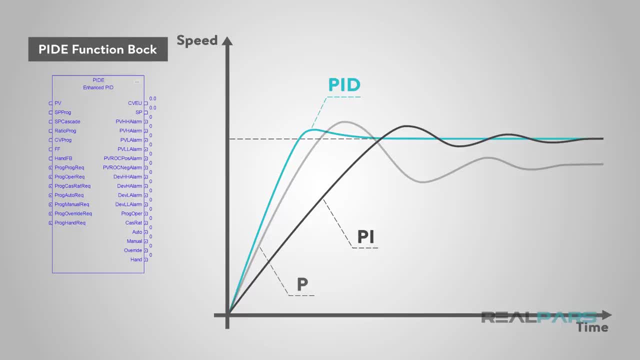 over the standard PID instruction for a few reasons. The PIDE instruction offers a built-in auto-tune feature which works reasonably well. The PIDE is programmed using a function block and not available for ladder logic programming. It uses the velocity form of the PID algorithm. 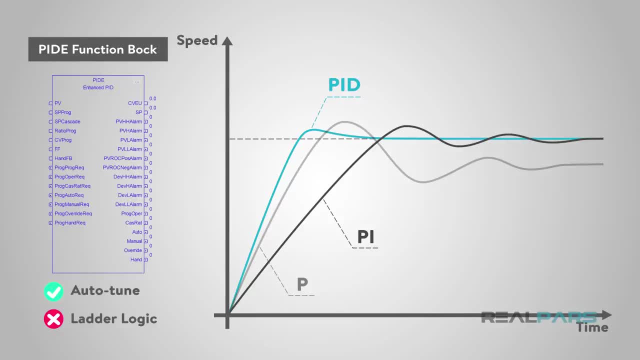 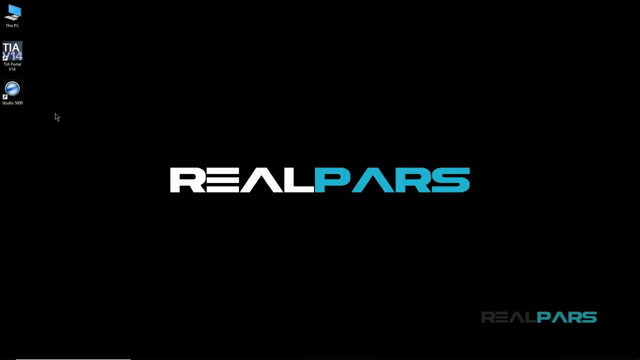 This is especially useful for adaptive gains or multi-loop and cascade process control. The PIDE instruction can be switched between program and operator modes and provides full, bump-less transfer into and out of cascade mode, and this instruction has more fault handling selections. The following programming steps assume the reviewer has Studio 5000 experience. 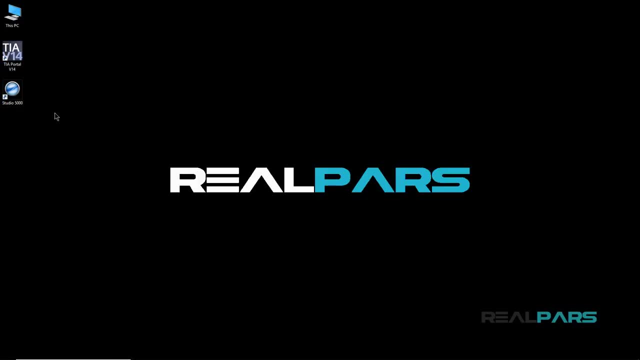 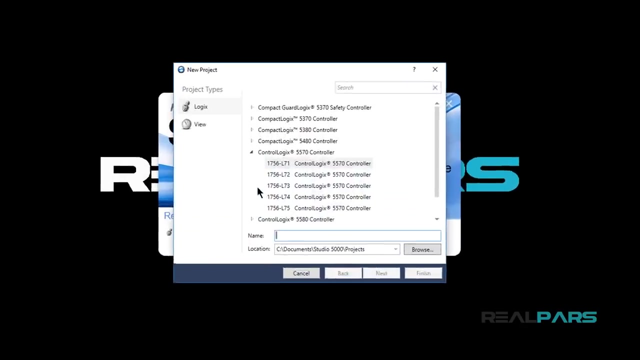 Ok, let's get started and create a new Studio 5000 project. Locate the desktop or taskbar icon for Studio 5000 and launch the program. Create a new project. Select a new controller type, such as the 1756L71,. 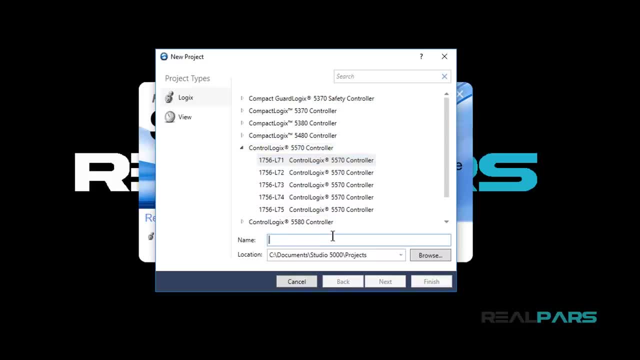 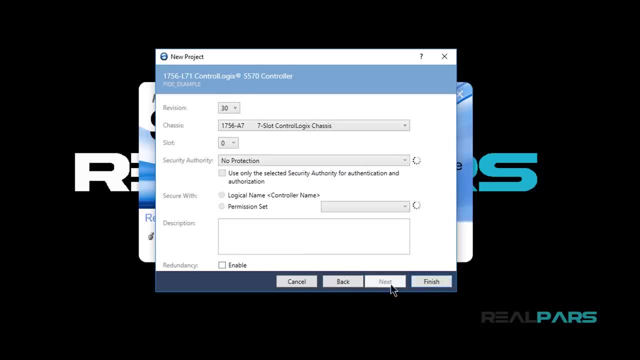 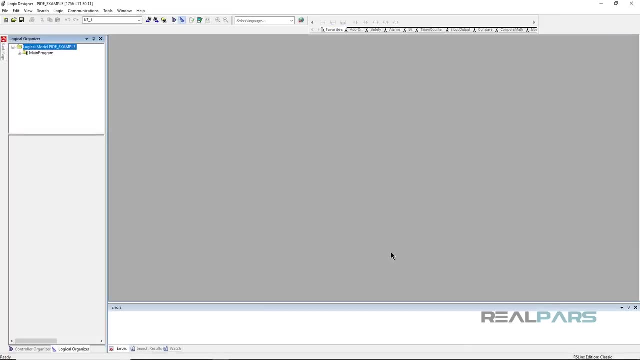 and select the new controller type. Select the 1756L71 and give the program a name, in this case PIDE. Example: Hit next and in the next window, keep everything as it is and then click finish. For the next step, we need to create a new routine by making a new task and a new program. 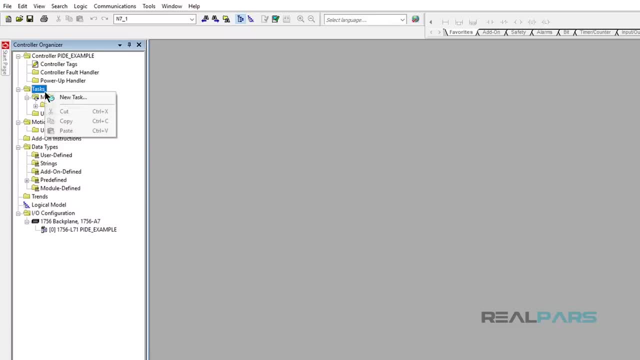 So first I'll create a new scheduled task by right-clicking on the tasks and then clicking on the new task In the next window. I will consider PIDE Control as the name for the task. The period of the task automatically becomes the sample rate of the PID loop. 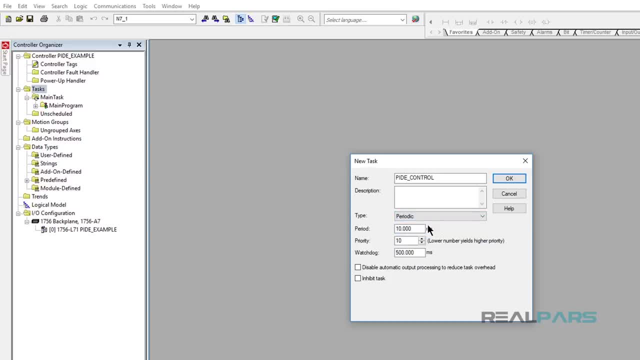 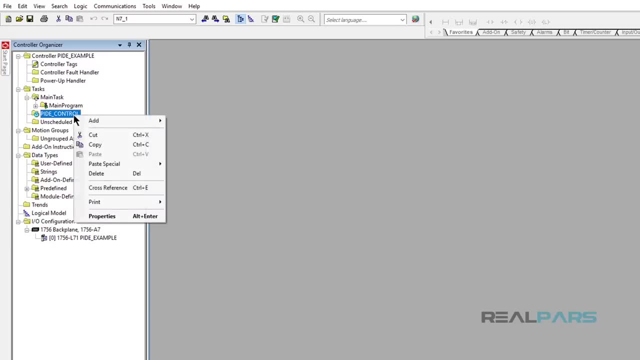 It is best to set it up in its own periodic task. So I'll leave these settings without any changes and continue to create a new program. by right-clicking on the PID Control task In this menu, I will open the Add Menu and click on the New Program. 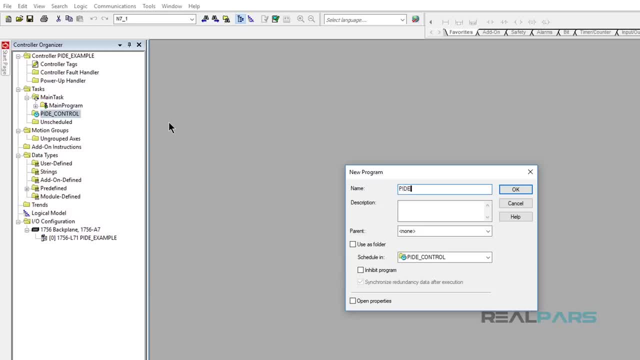 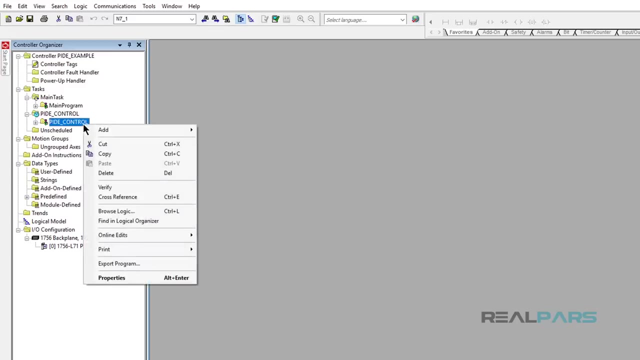 I will name the program the same as the task, which is PID Control. Finally, I will click OK to close this window. The next step in the process is to create a new routine. to do that, I'll right-click on PID Control program. 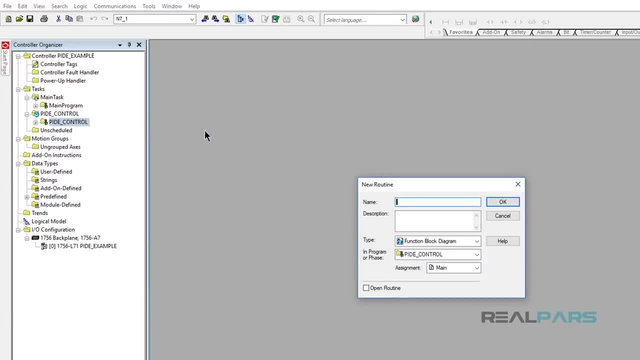 then Add, and then I will select New Routine. In this window. I will name the new routine as PIDE. Just make sure to select the type as function block diagram and then click OK. As you can see, the PIDE icon is added here. 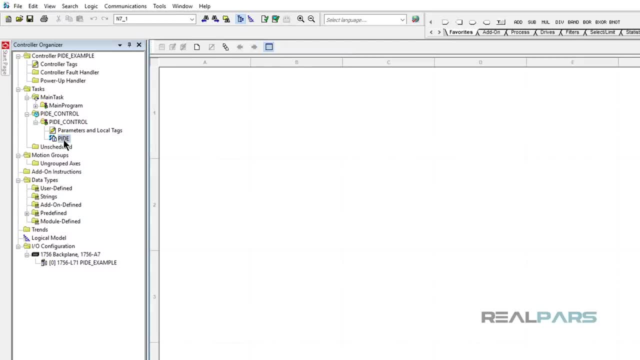 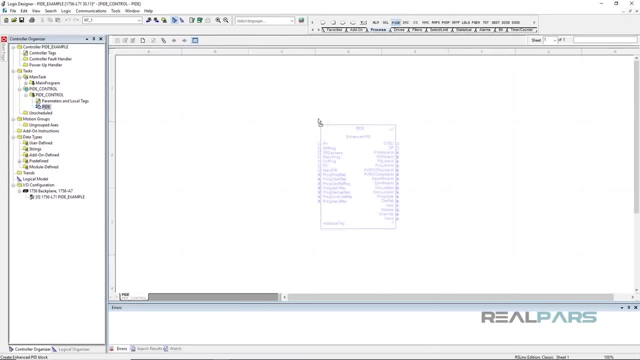 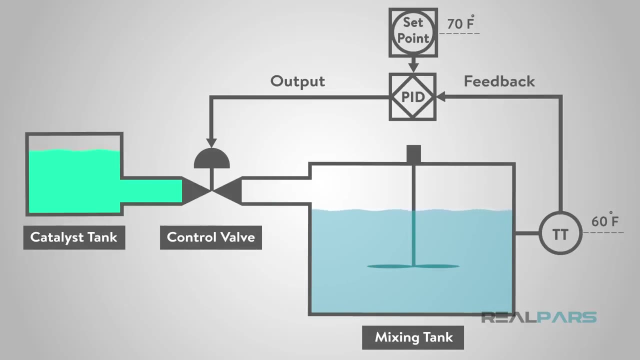 and I can open it up by double-clicking on it. Now that I have opened the PIDE program from the process tab in the library, I will add the PIDE function and add it to the sheet. Now let's suppose we have a mixing tank. 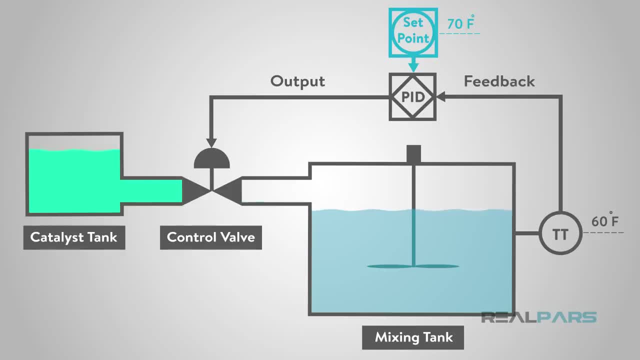 where the temperature is to be maintained at a certain setpoint. The control valve allows a catalyst to be added to the tank to increase the temperature, and the temperature transmitter will send the feedback to the PID. This will represent our process and control loop for programming purposes. 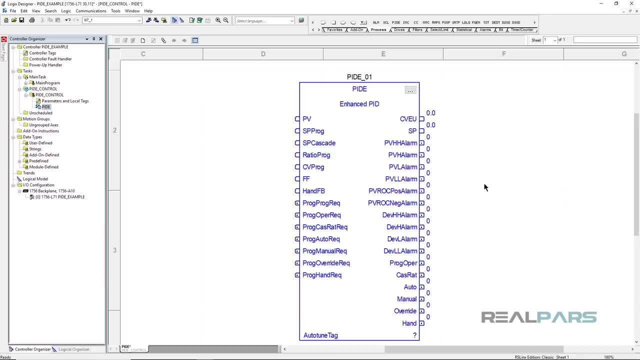 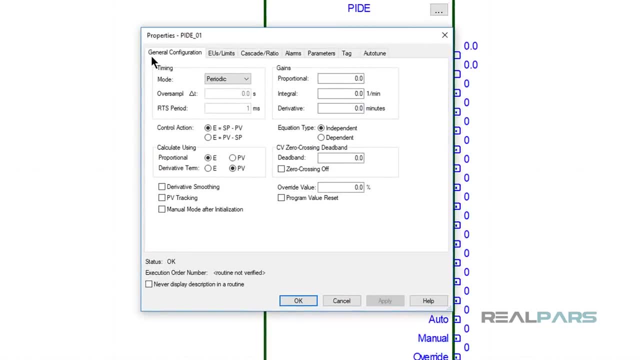 Now, to be able to configure this block, I need to open up the properties. To do that, I'll simply double-click on the block In the General Configuration tab. we will use the default configuration. However, we just need to make sure that, for the timing, it is using periodic mode. 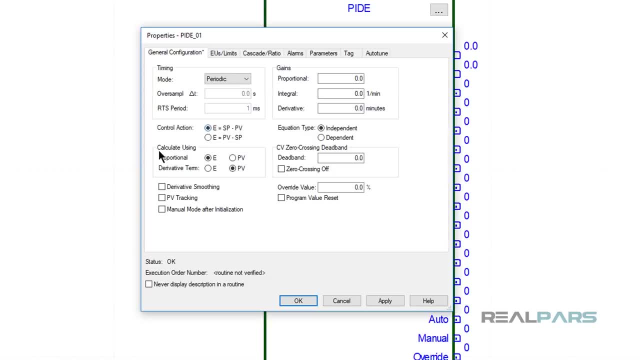 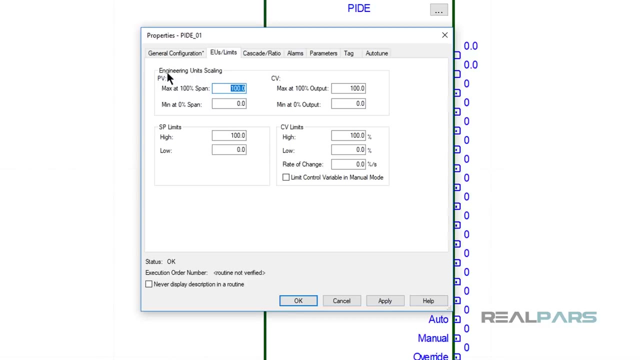 The control action is set to E and for the calculate it is using the proportional parameter Set to E and the derivative term is set to PV. Next, in the EU's Limits tab, I will set the engineering unit scaling for both CV and PV parameters from 0 to 2500 degrees Fahrenheit. 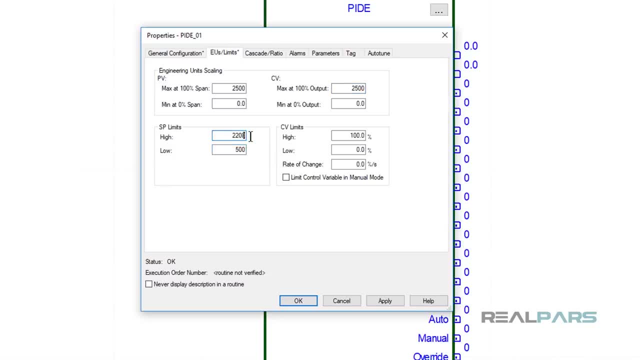 with a setpoint limit of 500 to 2200 degrees Fahrenheit, The control variable limits will be using the same temperature. The control variable limits will be using the same temperature as the engineering units. In the Parameters tab there are several parameters which PIDE function utilizes them. 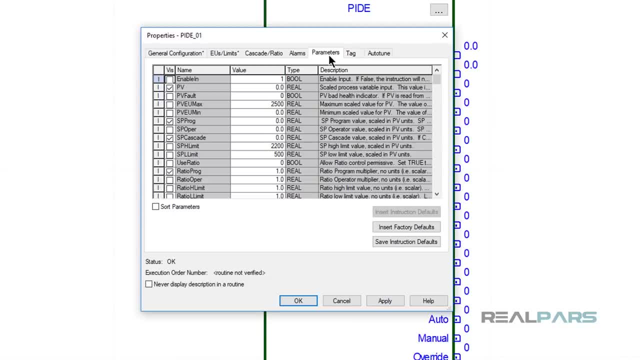 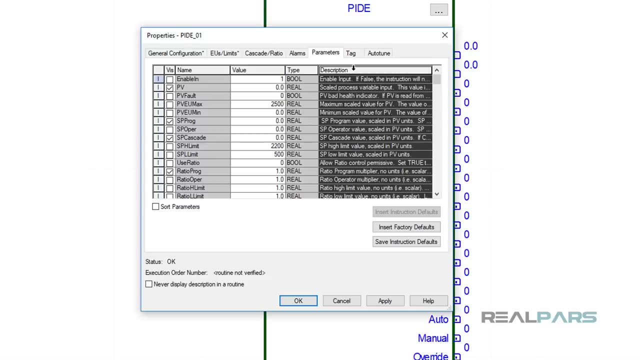 that you may or may not use them. These parameters can be manually turned off or on. here, When selected, the parameter will be exposed to allow program connections. Here there is also a description field for each parameter which gives you more information about them. 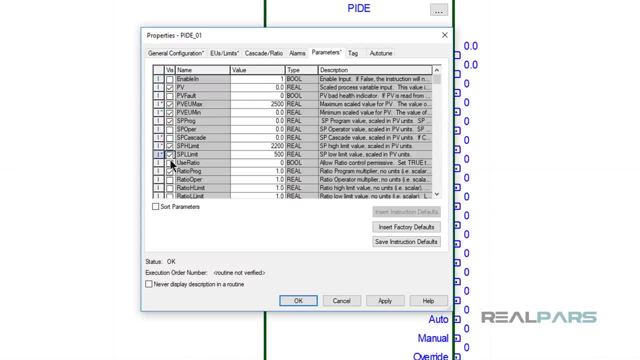 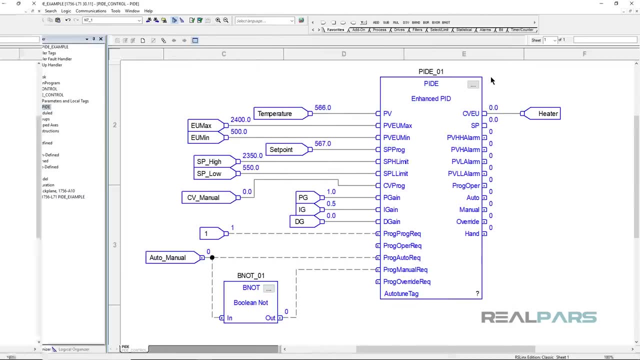 I'll select the required parameters and deselect the rest. Next I'll hit OK to save the configuration. You can see the required parameters I've selected in the PIDE block here. After the PIDE function block is configured, we can begin to add program control input and output reference tags. 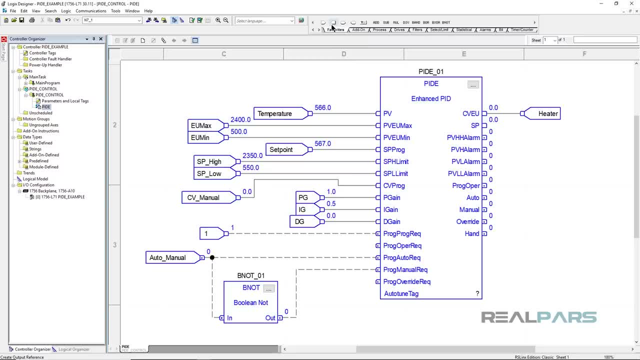 to adjust the PIDE block performance. The main input references are the temperature PV or process variable, which is a feedback from temperature transmitter, the SP-PROG, or program setpoint, which is defined by the operator on the HMI, and the CVEU, or control value and engineering units output. 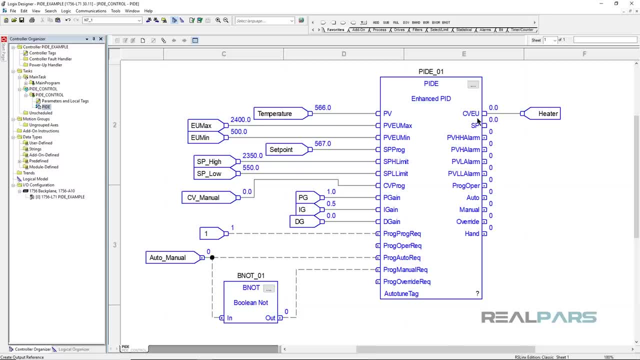 to control the heat in the tank by opening or closing the control valve. Other inputs added are inputs for controlling the setpoint, high and low limits, the maximum and minimum engineering units and auto manual control to allow for direct manual control of the catalyst control valve. 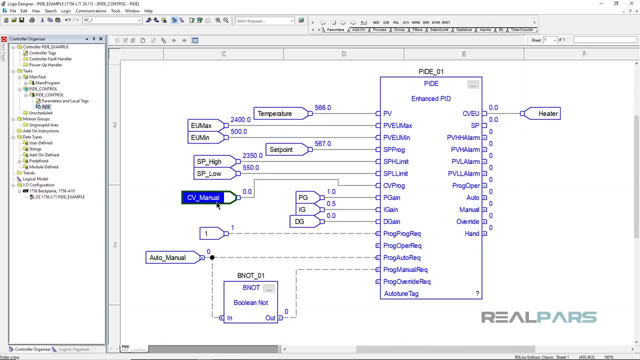 The CV manual input reference value will be used for the manual control when auto manual is turned off. The PIDE will need to be tuned and we have to set the tuning parameters: P gain to 1,, I gain to 0.5, and D gain to 0.5. 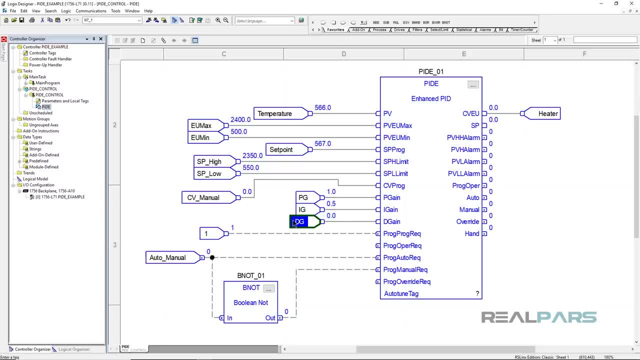 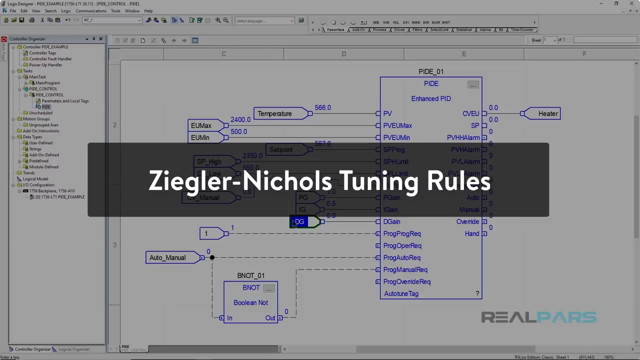 and D gain to 0 to a recommended starting point. PIDE tuning can be tricky, so I recommend reviewing procedures for this technique. The standard reference for PIDE tuning seems to be the Ziegler-Nichols tuning rules. This concludes the video. 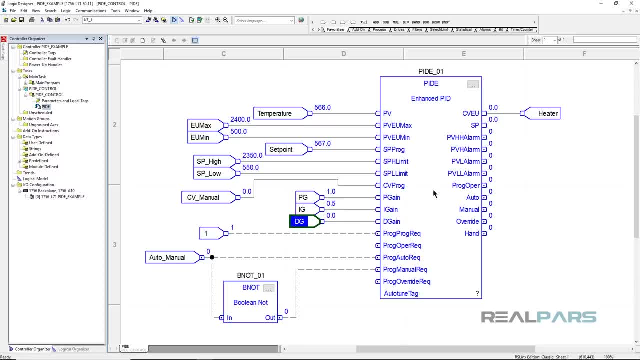 Programming: Basic Control Logics: PIDE Loop using the PIDE block instruction. I hope you've enjoyed learning what will support you in your upcoming project. If you would like to get additional training on a similar subject, please let us know in the comment section. 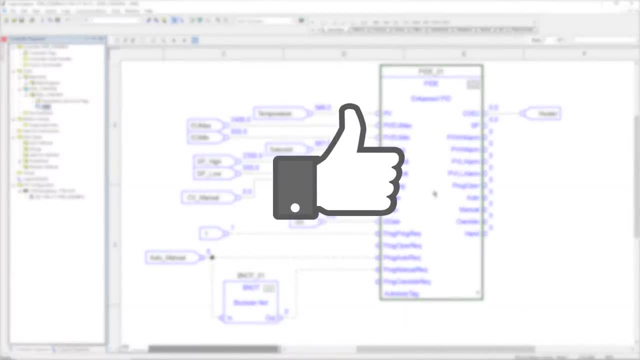 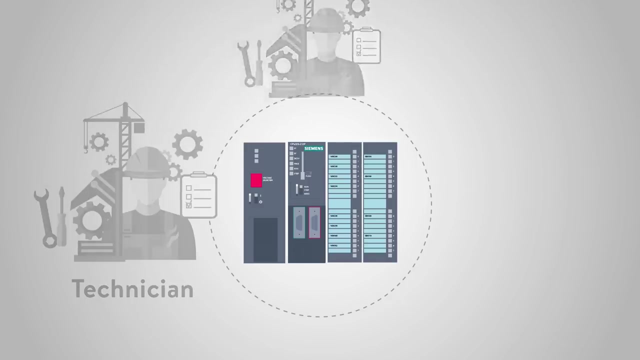 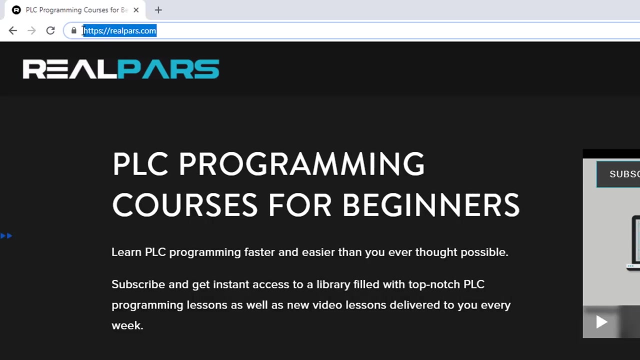 If you enjoyed this video, please press the like button. Please check back with us soon for more automation control topics. Want to learn PLC programming in an easy to understand format and take your career to the next level? Head on over to realparscom.